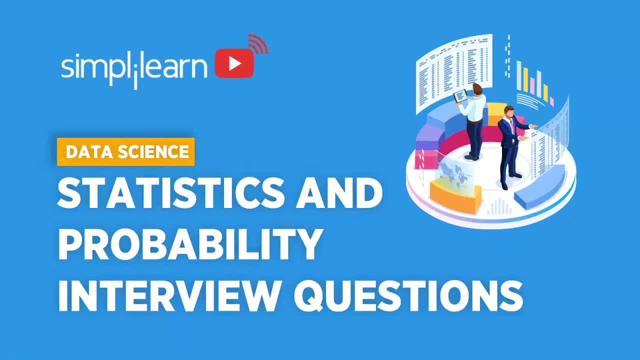 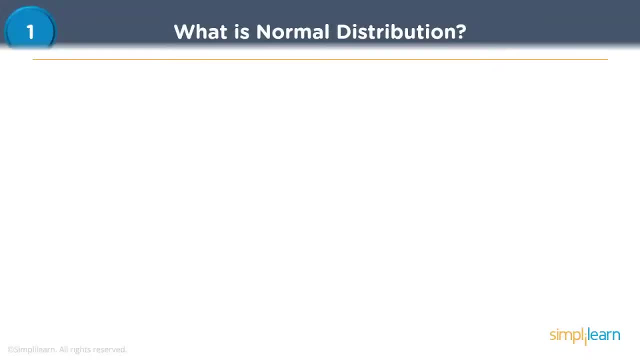 If you have any questions, then please feel free to put them in the chat section of the video. Our team will help you solve your queries. So let's begin with our first question. The first question we have is: what is normal distribution? 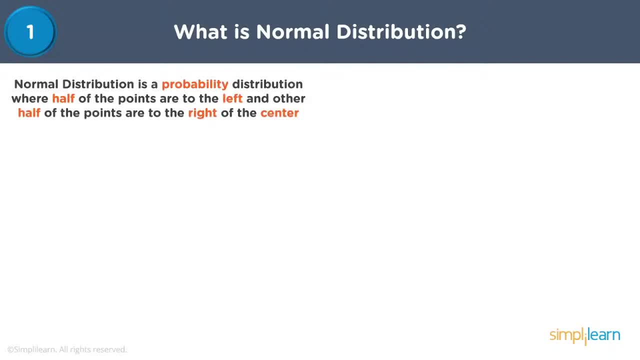 Now, normal distribution is a probability distribution that is used to check how your data is distributed. Your data could be spread out to the left or to the right, But in many cases the data tends to be around a central value, with no bias left or right, as you can see on your screens. 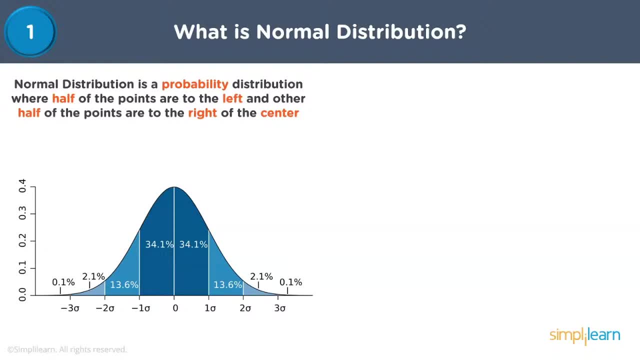 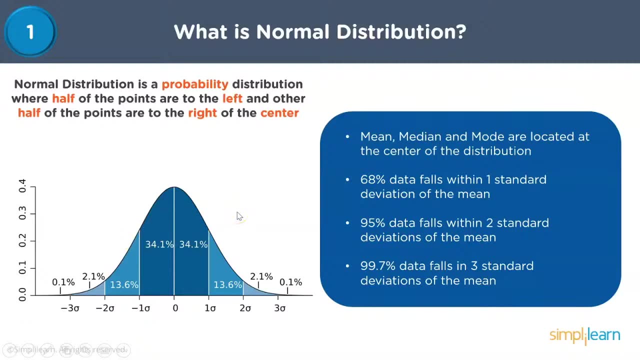 Now this is called a normal distribution, where half of the points are to the left and another half of the points are to the right of the center. Now such a distribution contributes to 68% of the data. This means that the data is falling within one standard deviation of the mean. 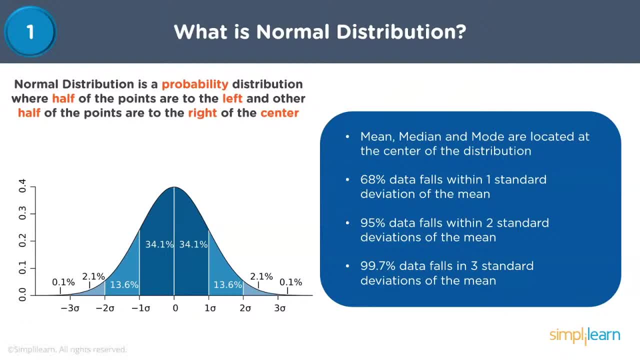 Then we have 95% of the data falls within second standard deviation of the mean. So if you add up 13.6% and the 68% plus 13.6%, this will result to 95% of data falling within two standard deviations of the mean. 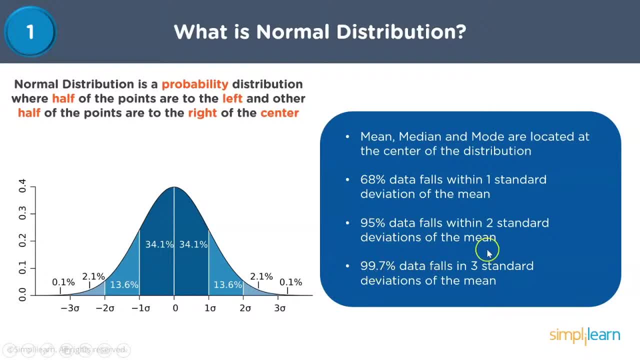 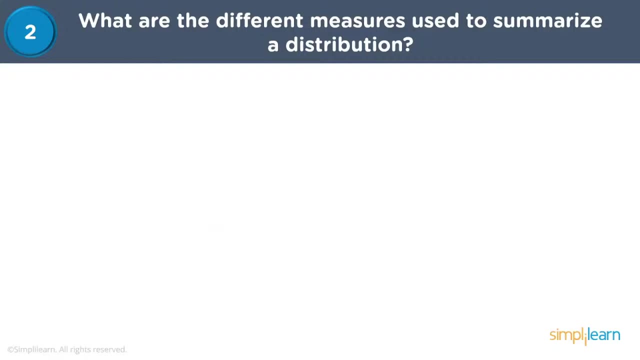 And, finally, we have close to 99.7% of the data falling within three standard deviations of the mean. So this is what a normal distribution is all about, Number two, Moving on to the next question. So what are the different measures that are used to summarize a distribution? 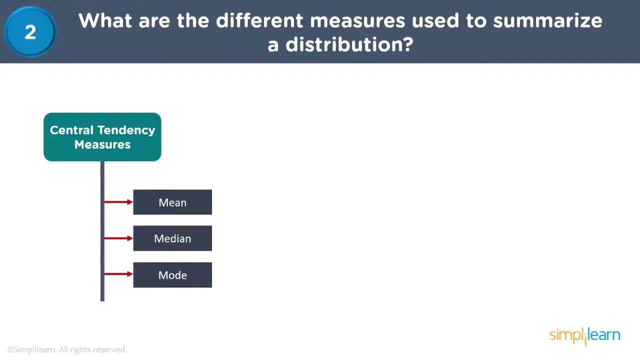 Now, to get more idea about the data and summarize a distribution, you can use three types of statistical measures. The first, we have central tendency measures. Then we have variation measures And finally we have shape measures. Now, under central tendency measures, we have mean, median and mode. 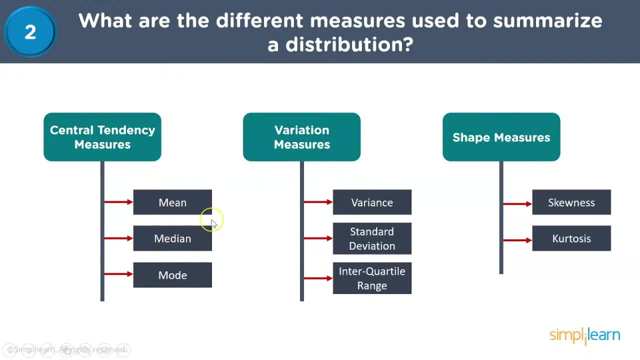 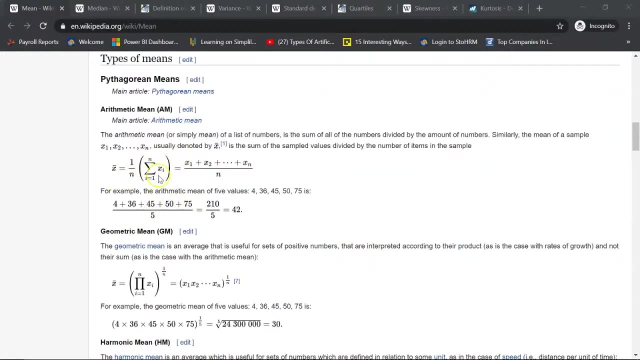 Now the mean is the most frequently used measure of central tendency In a data set. let me take you to the Wikipedia page and explain you what mean exactly is Okay. So here you can see on the Wikipedia page. it has the formula to calculate the mean of a distribution. 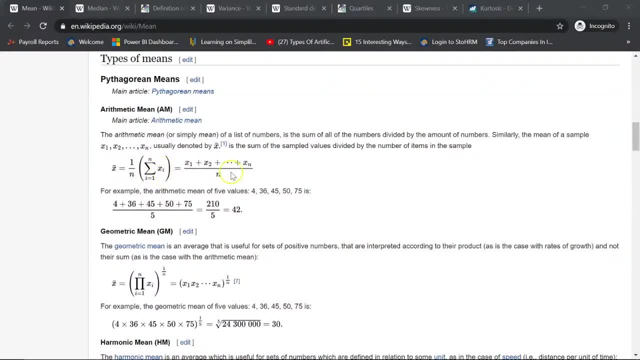 So this is basically the summation of all the data points divided by the total number of data points. So here you can see an example. We want to find the arithmetic mean of five values which are 436.. We want to find the arithmetic mean of five values which are 436.. 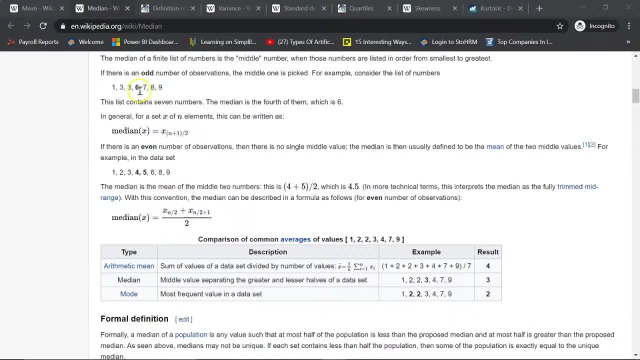 So we want to find the arithmetic mean of five values, which are 436.. We'll pick the fourth element from our ordered set of points. that is six here, And hence six is the median for this ordered set of points. Now, if you have an even number of observations, as you can see here, total we have eight observations. 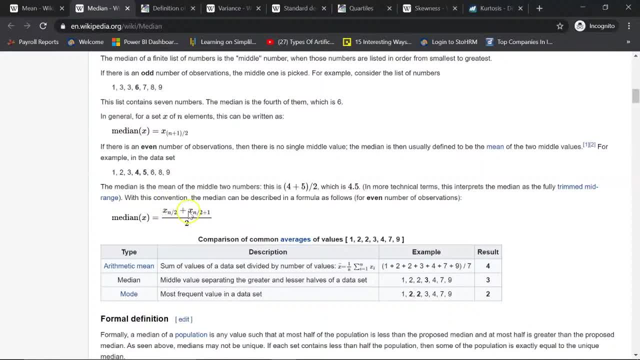 Now the median becomes xn by 2 plus xn by 2 plus 1 divided by 2.. So your median becomes the mean of the middle two numbers, that is, 4 plus 5 by 2, which is 4.5. 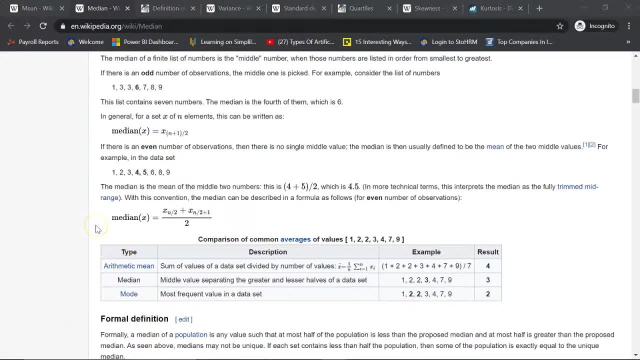 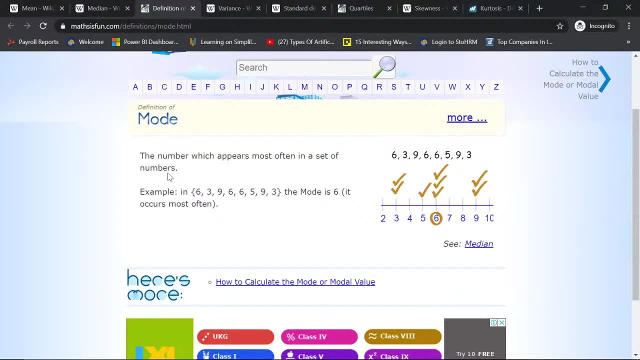 All right Now. the next statistical measure we have under central tendency is called the mode. So the mode is the most frequently occurring value in a set of data points. So here you can see an example. We have a set of data points: 6,, 3, 9,, 6,, 6,, 5,, 9,, 3.. 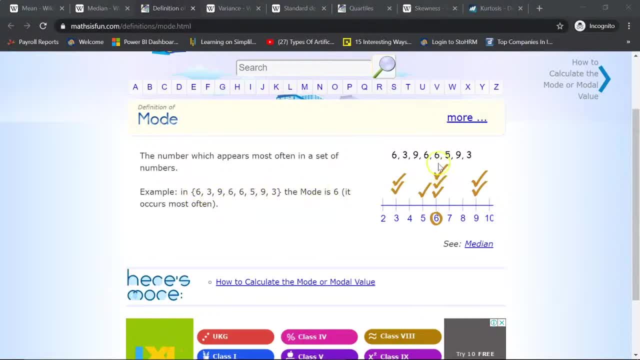 So your mode is going to be 6 here. Since 6 is occurring, This code needs to be used to define xth, ie. it's going to be h included here, And so in this room, from here in the node noise convention. 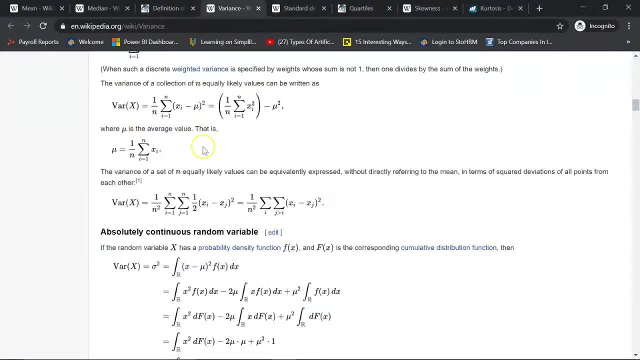 One set of data points. Now, here we want to say that the information for the knowledgeed these set of data points is xn �. Next step, we're going to call this sequence. So the quota bar in this skinnyızı here, this is the data data bar. 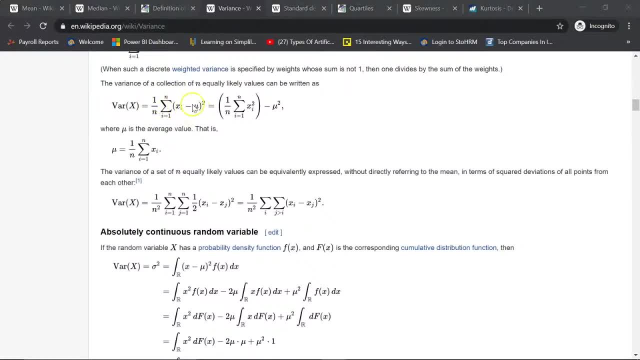 Y using what we're going to call this ket, 就是 a value of x in this set of data points, And we will take this and make it spot: the summation of all the data points divided by the total number of data points. so this is your. 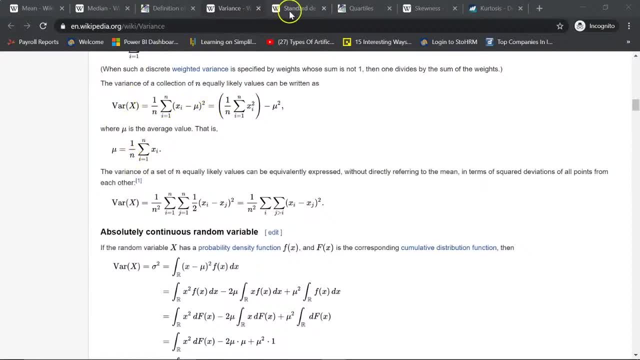 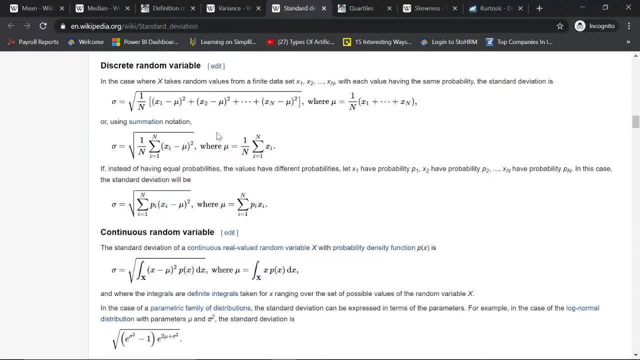 formula for variance. next we have standard deviation. so standard deviation is a measure of the amount of variation or dispersion of a set of values. a low standard deviation suggests that the values tend to be close to the mean, while a high standard deviation suggests that the values are very spread out. now, here you can see the formula for variance. now this is denoted. 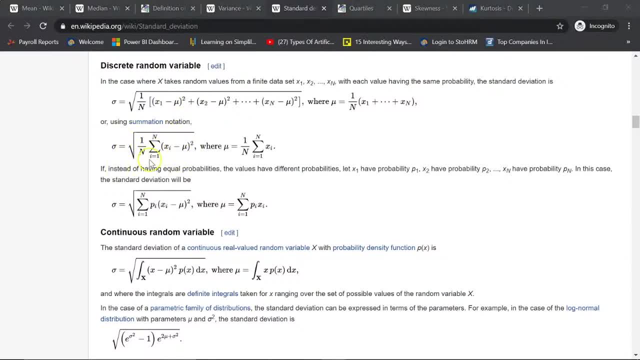 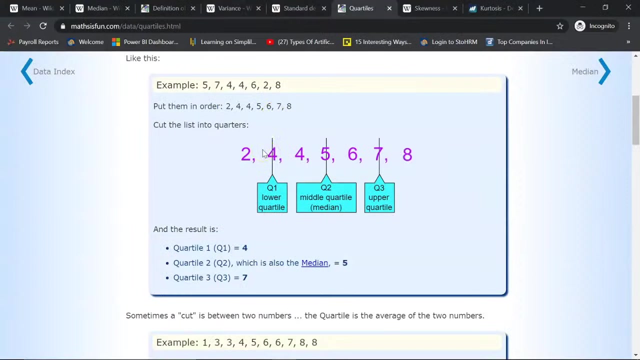 by sigma, and your standard deviation is nothing but the square root of variance. so here you can see the formula for variance: your xi minus your mu square, which is the mean of all the data points divided by n. then we have the interquartile range, which is also known as iqr. so iqr is a measure of. 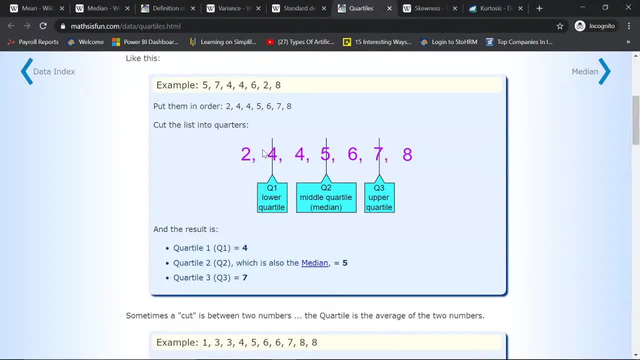 variability based on dividing a data set into quartiles, so an interquartile range range measures where the bulk of values lie. so the formula for IQR is q3, which is the third quartile minus the first quartile. so here you can see, we have a. 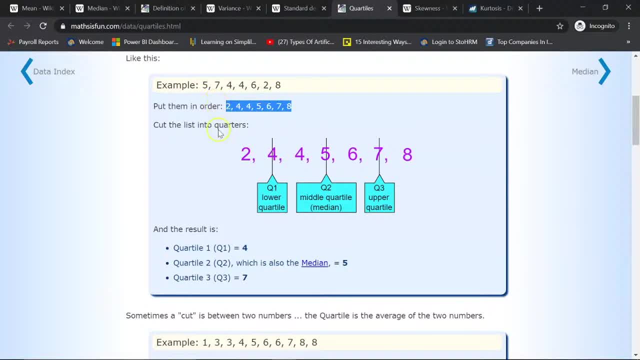 list of data points. then we are ordering the data points first and then we cut the list into quarters. so first you have the q1, then you have q2 and finally you have q3. so for these set of data points your IQR is going to be 7 minus 4. that 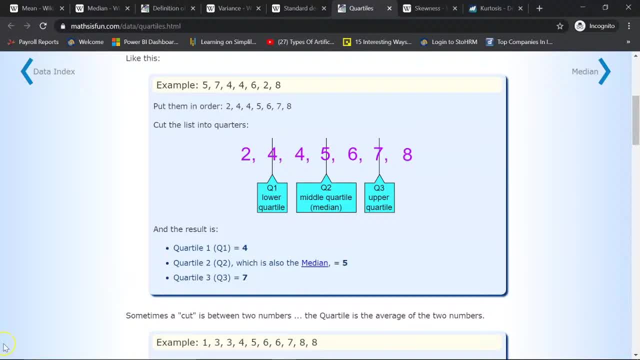 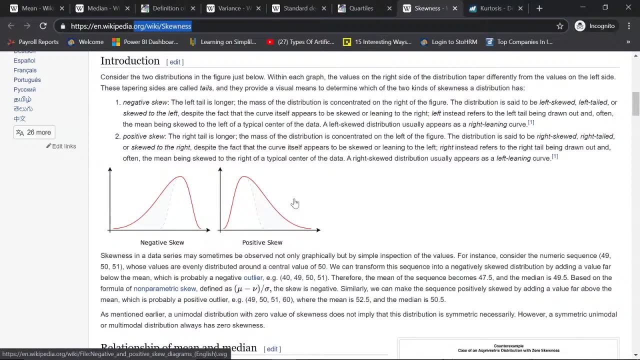 is 3. then we have shape measures. so under shape measures we have skewness and cotosis. so skewness is a measure of symmetry. your distribution is symmetric if it looks the same to the left and the right of a center point. now they are majorly of two types. one is called 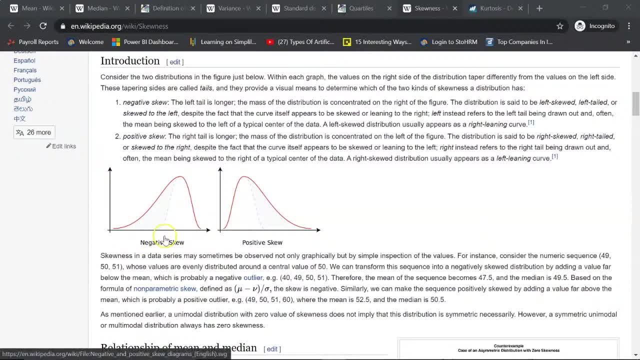 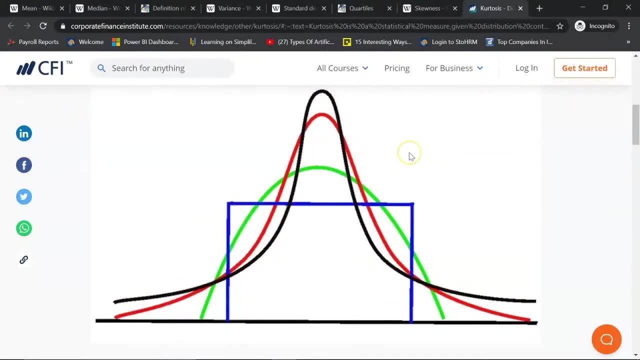 Q3 and the other is Q3. so for these set of data points, your IQR is going to be negative skew, or which is also known as left skew, then we have positive skewed or right skewed and finally we have cotosis. so cotosis is a measure of the 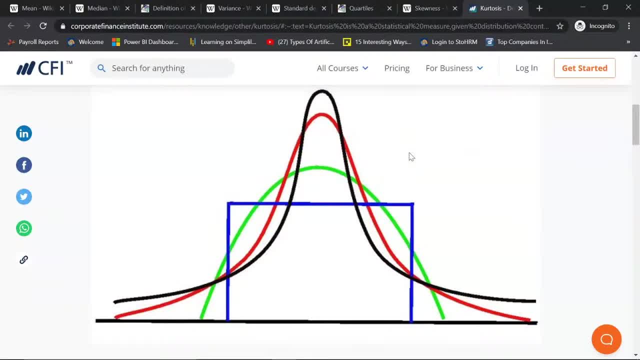 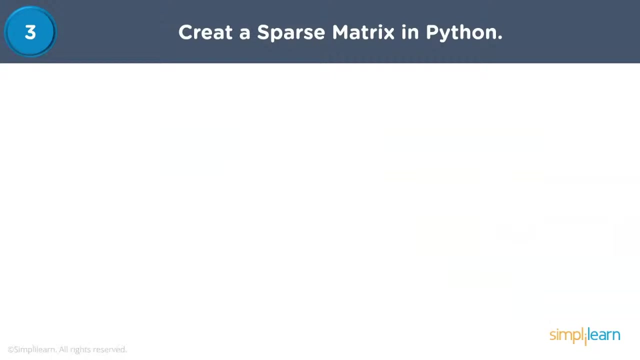 tailedness of a probability distribution. it defines how heavily the tails of a distribution differ from the tails of a normal distribution. so if you consider these distributions, the cotosis will calculate the tailedness which is actually these areas of a distribution. now let's look at a third question. so the question is: create a sparse matrix in. 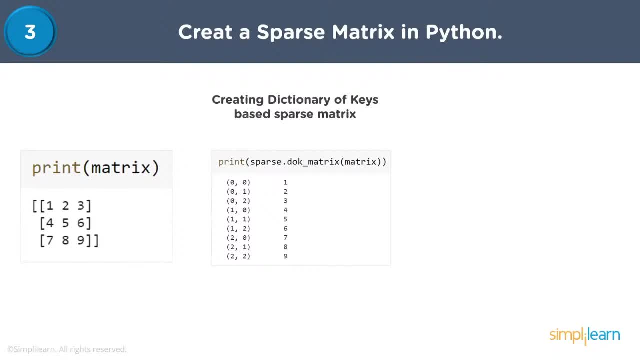 Python. now in numerical analysis, a sparse matrix or a sparse array is a matrix in which most of the elements are 0. there are multiple ways to create a sparse matrix. I'll show you two ways to create a sparse matrix. so let me take you to my Jupyter notebook, where I'll create a matrix first and then we'll see how to. 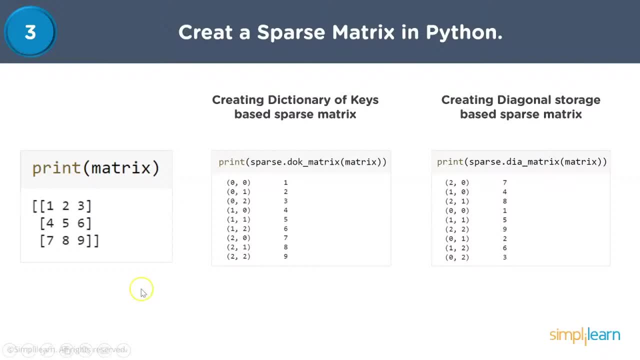 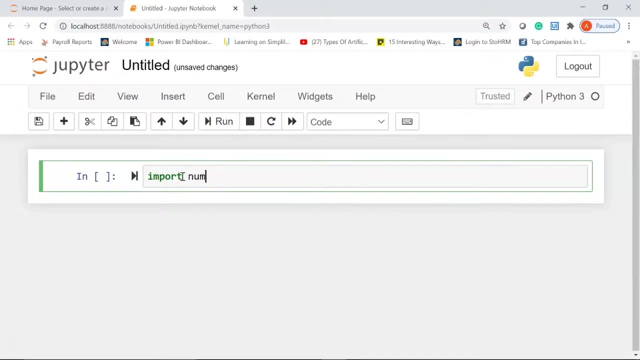 create sparse matrix out of it. so I am on my Jupyter notebook here. first let me import the necessary libraries. so first I am going to import numpy as NP, and then from scipy we'll import sparse. I'll run this cell, okay. next let me go ahead and create a. 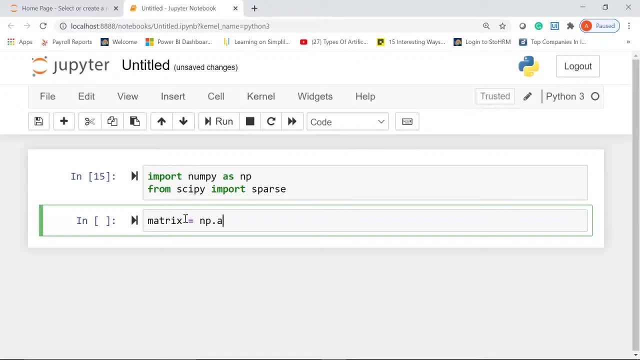 matrix. I'll use the NP dot array function and within this function I'll create a 3 cross 3 matrix and I'll assign the elements. so my first row will have 1, 2, 3, next we'll have 4 comma, 5 comma, 6, then we'll have 7, 8 & 9. 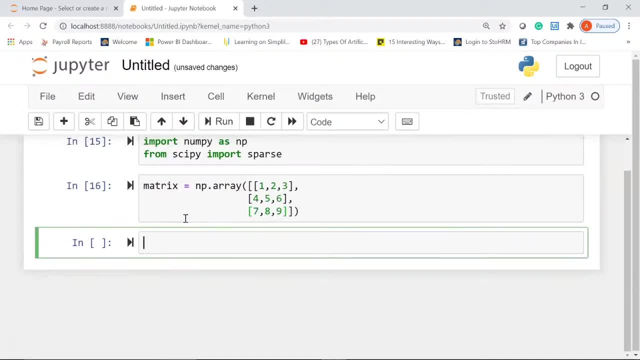 all right, let me run this cell. okay, now let me go ahead and print my matrix. so I'll use the print function and let's say, I'll pass in a message that is original matrix comma and then pass in my variable name that is matrix. let's. 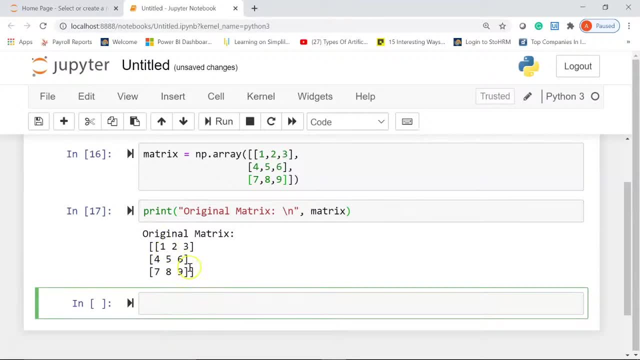 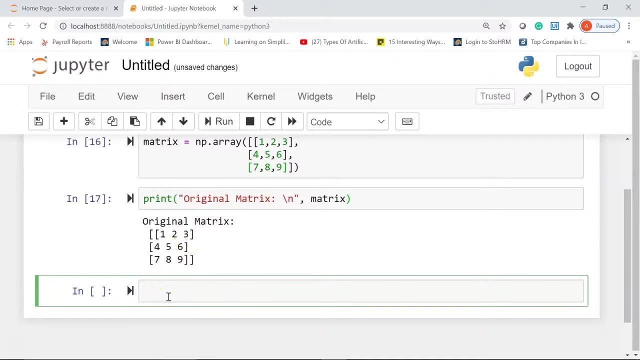 run it. so here you can see I have my original matrix. it is a 3 cross 3 matrix and has 9 elements in it. first let's see how, using dictionary of keys, you can create a sparse matrix. so for that I'll write the print statement and. 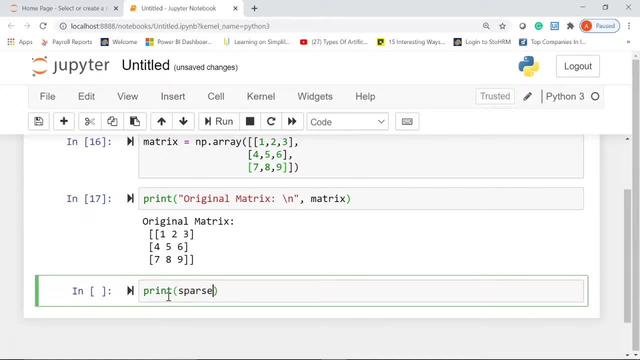 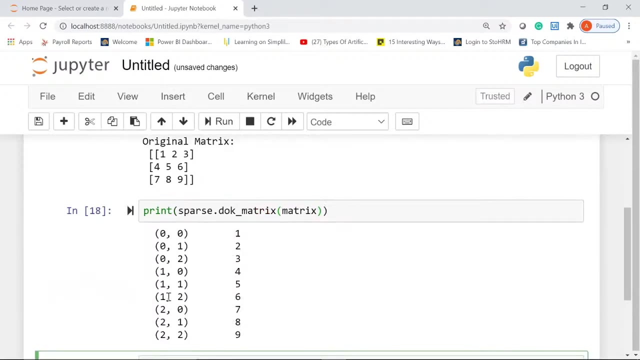 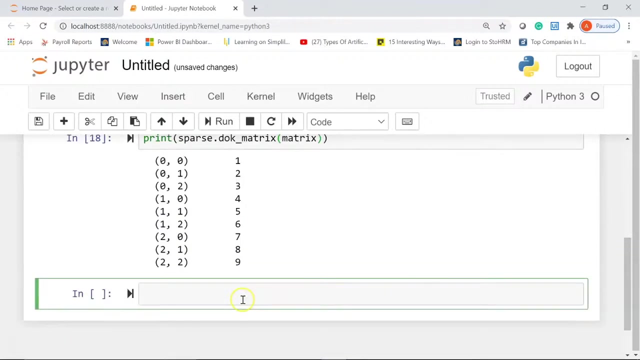 then I'm going to use a function which is called DOK- that stands for dictionary of keys, underscore matrix, and I'll pass in my variable name which is my original matrix. so if I run this you can see I have got my dictionary of keys, sparse matrix. next I'll show you. 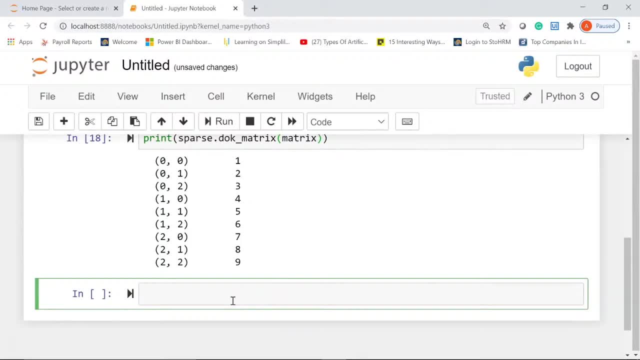 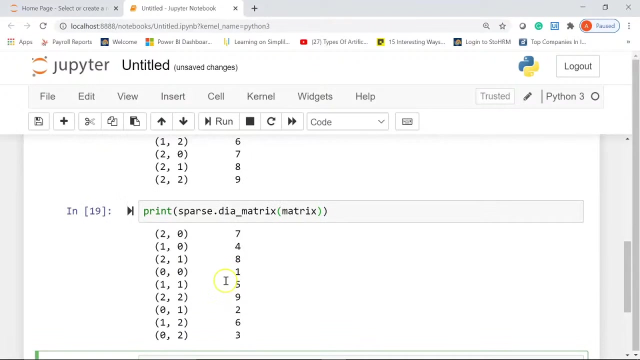 how, using diagonal storage paste, you can create a sparse matrix. so this is an example, so you can see that you can create sparse matrix. next I'm going to use another function, that is sparse dot dia, which stands for diagonal underscore matrix, and within this function I'll pass in my original matrix variable name. if I run this, you can see we have. 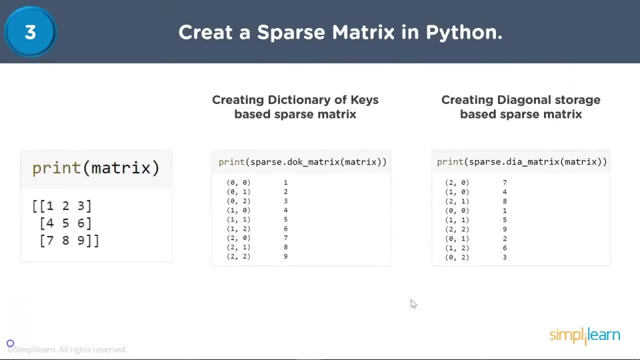 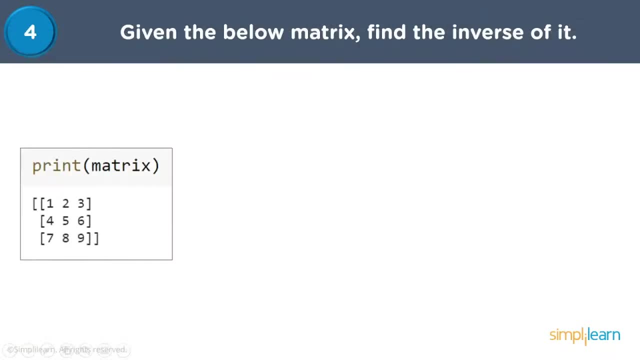 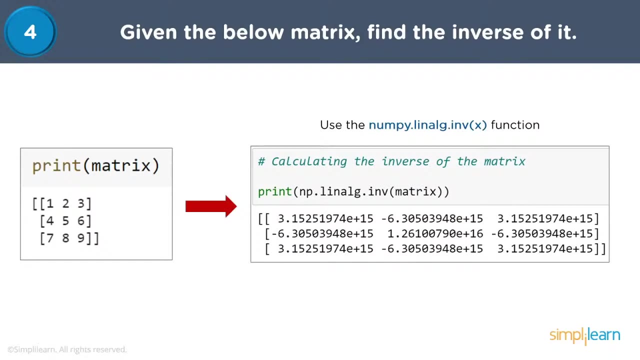 Now moving to the next question. So given below is a matrix. Now we need to find the inverse of this matrix. Now the inverse of a square matrix A, which is sometimes called as a reciprocal matrix, is a matrix, A inverse, such that the dot product of A and A inverse. 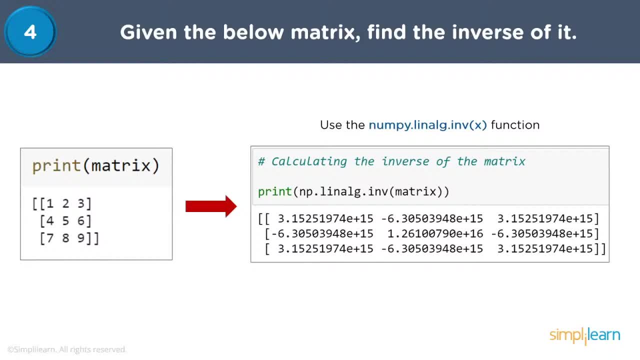 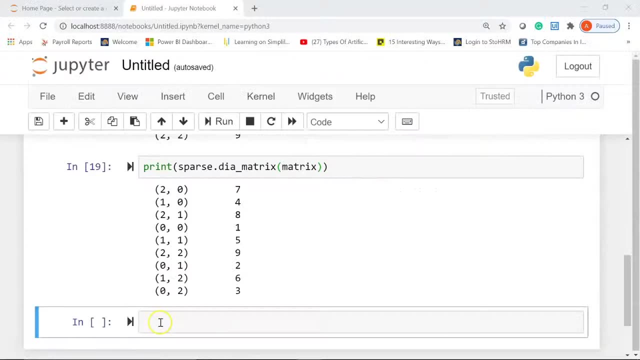 is always I, which is an identity matrix. Now in NumPy we have a function which you can see here, that is nplinalginv. that helps you find the inverse of a matrix. Let me show you on the Jupyter Notebook. First let me print my original matrix. All right, 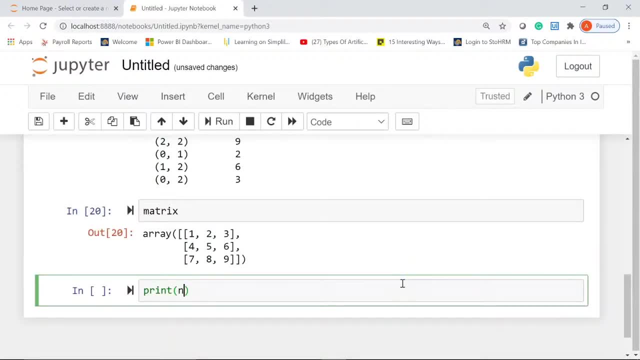 Now here I'll use the function with min, that is nplinalginv, which stands for inverse, And then pass me my variable name, that is matrix. If I run this, you can see I've got the inverse of my original. 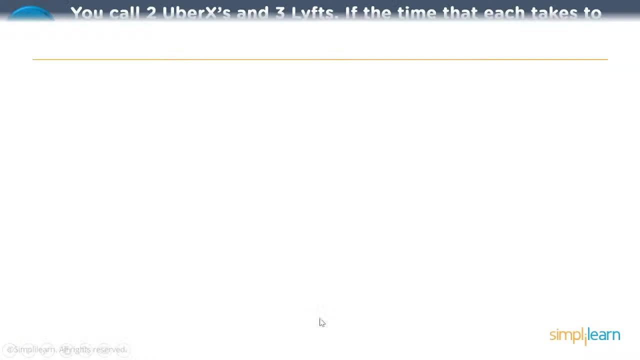 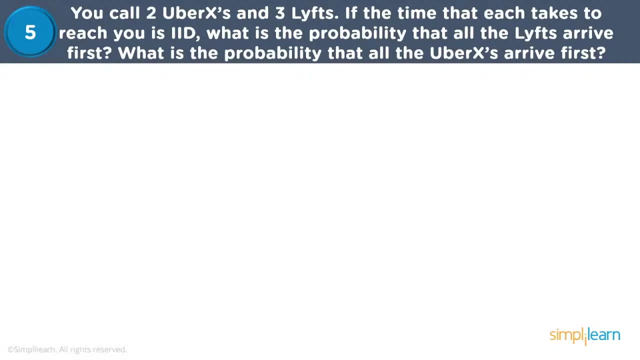 matrix. Now moving to our fifth question. So this question is related to probability. You call two UberX and three Lyfts. If the time that each takes to reach you is IID, what is the probability that all the Lyfts arrive first? Next, we want to find what is. 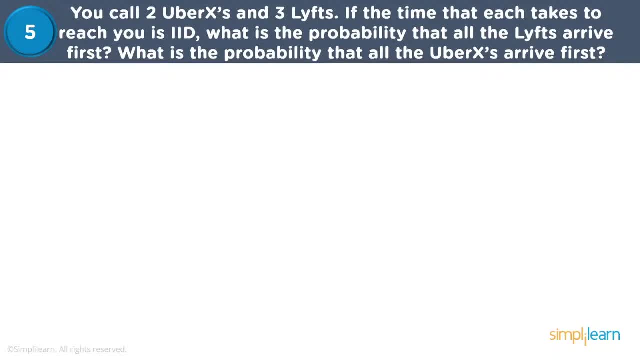 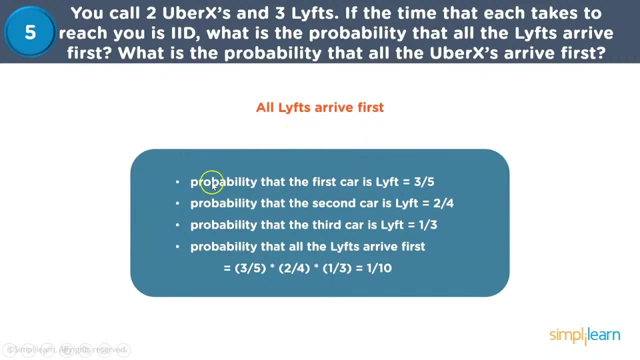 the probability that all the UberX arrive first. Now, this is fairly a simple question. First, let's look at how the Lyfts arrive first, Then. first we need to find the probability that the first car is a Lyft, which is going to be 3 by 5, since we have three. 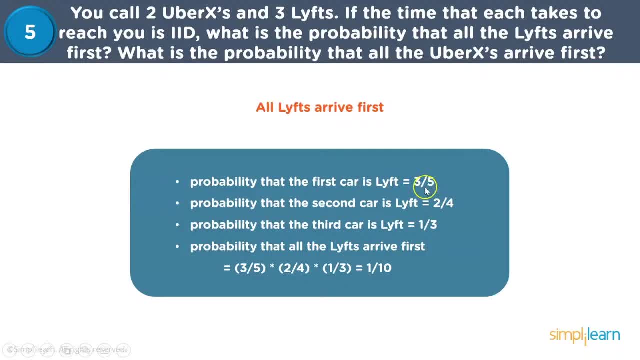 Lyfts and total, we have five vehicles. Next, we want to find the probability that the second car is a Lyft, which is going to be 2 by 4.. Third, we need to find the probability that the third car is also a Lyft, which is 1 by 3.. Now let's arrive. 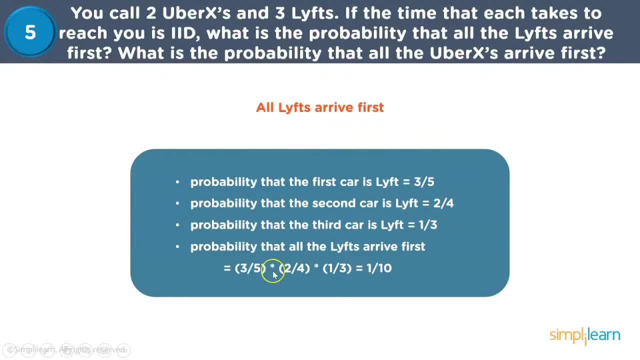 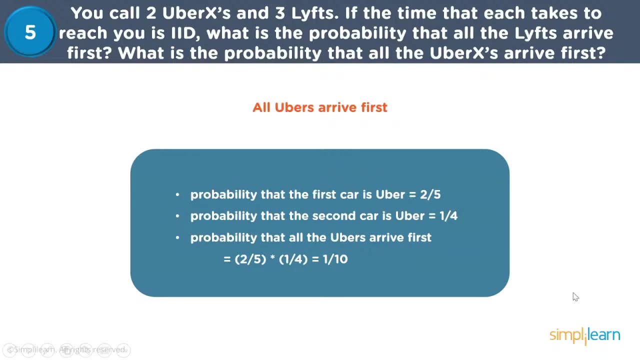 first is going to be the multiplication of the product of the above three probabilities, that is, 3 by 5 into 2 by 4, into 1 by 3, which is nothing but 1 by 10. next, let's say you want to find for all the Ubers that arrive first. so you need to find the probability. 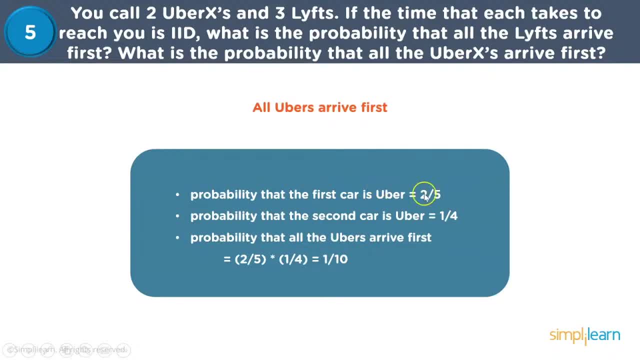 that the first car is Uber, which is nothing but 2 by 5, since we have two Ubers. next, the probability that the second car is an Uber is going to be 1 by 4. so the total probability that all the Ubers arrive first is going to be the product of 2 by 5 and 1 by 4, which 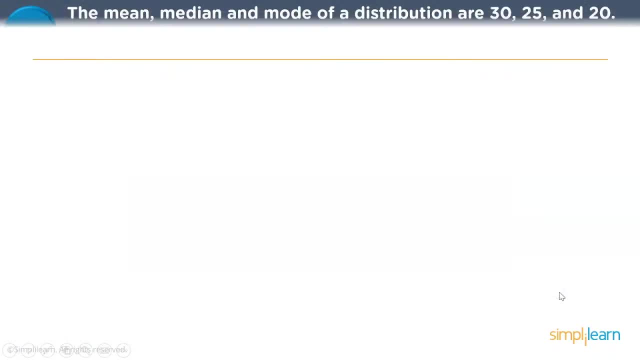 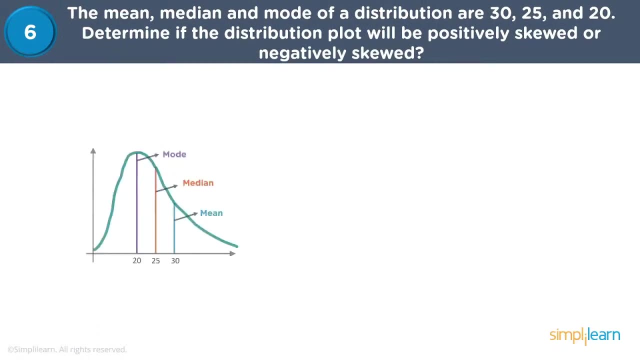 is also 1 by 10. now moving to the 6th question. the mean median and mode of a distribution are 30, 25 and 20. we need to determine if the distribution plot will be positively skewed or negatively skewed so you can see. see if the distribution plot is positively skewed or negatively skewed, so you can see. 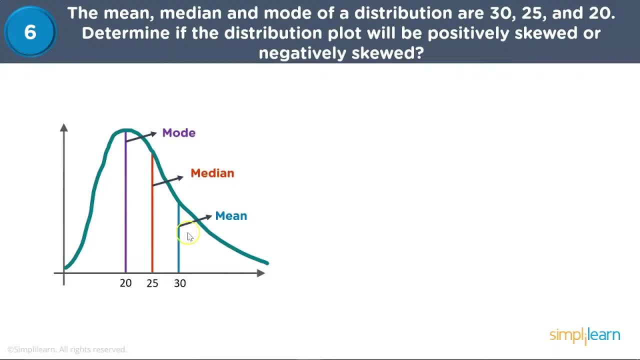 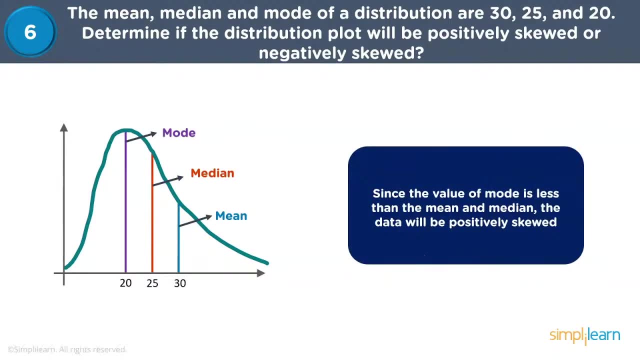 if the distribution plot is positively skewed or negatively skewed. so you can see from the distribution graph, the mean is to the right, median to the middle and mode to the left. so since the value of mode is less than the mean and median, the data will be positively skewed and similarly the skewness of the distribution is on the left if the 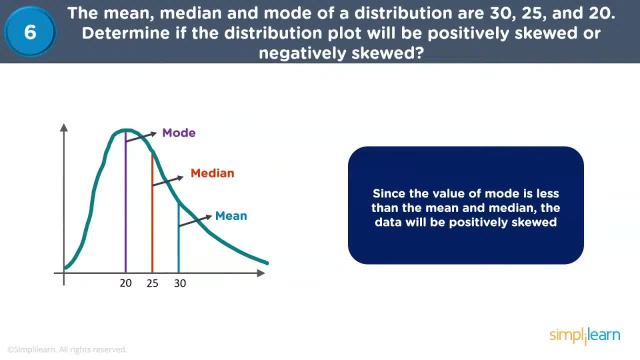 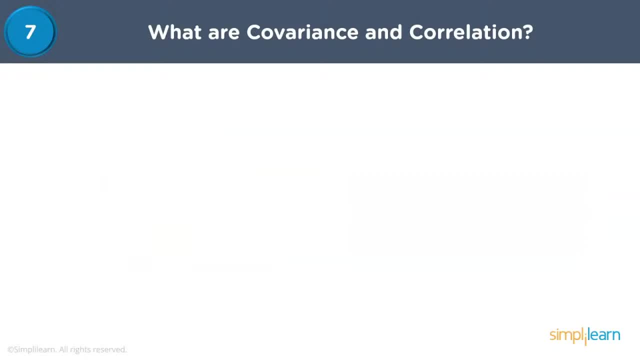 mean value is less than the median and the mode occurs at the highest frequency of the distribution. now the next question we have is: what are covariance and correlation? so covariance and correlation are measures that help you understand the relationship between two continuous variables. so covariance tells the direction of the linear relationship between. 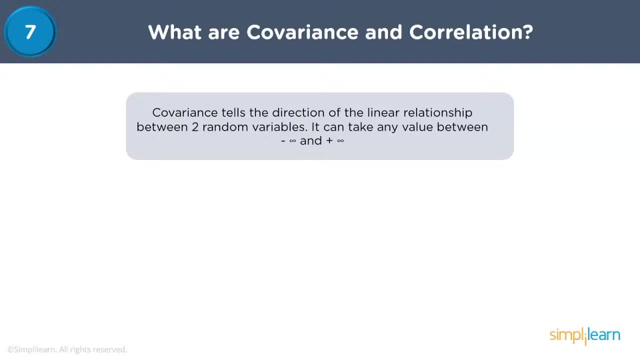 two random variables. the direction means if the variables are directly proportional or inversely proportional to each other. so increasing the value of one variable might have a positive or a negative impact on the value of the other variable. now covariance can take any value between minus infinity and plus infinity. so below you can see the formula to calculate. 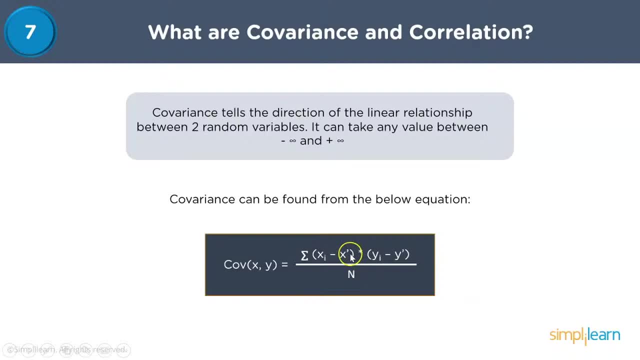 the covariance. so you have summation: xi minus x bar. x bar or x dash here represents the mean, xi represents the individual points. then this is multiplied by yi minus y dash, or the mean of y divided by the total number of observations. next we have correlation. so correlation explains. 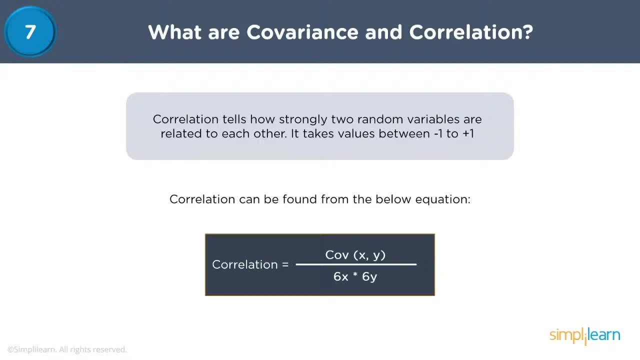 the correlation of the number of observations. so correlation explains the number of observations. change in one variable leads to how much proportion changes in the second variable. correlation tells how strongly two random variables are related to each other. it takes values between minus one and plus one. a negative correlation means they are inversely proportional to each. 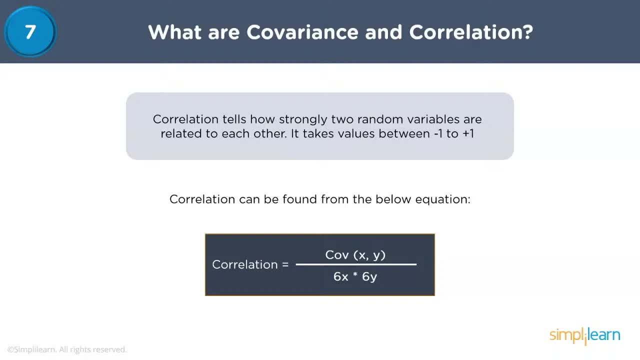 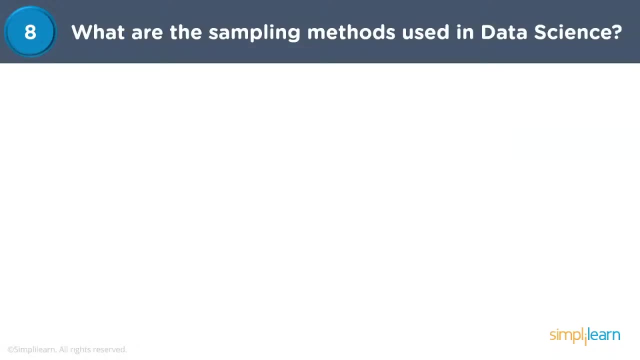 other. a positive correlation means they are directly proportional to each other. if the correlation coefficient is zero, then there is no linear relationship between the variables. so here below you can see the formula to calculate the correlation. Now moving on to the eighth question. so what are the sampling methods used in data science? 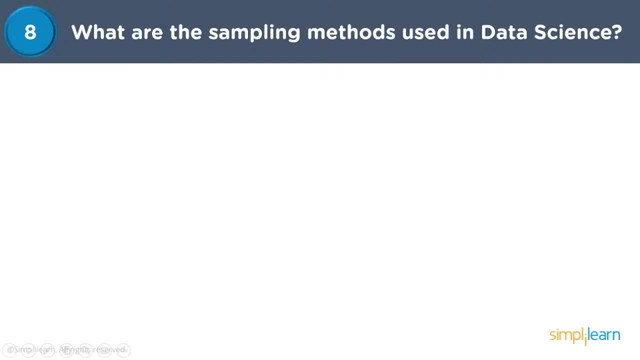 now, sampling is a statistical technique that is used to select, manipulate and analyze a subset of data points and find patterns and trends in the large data set been examined. now there are two types of sampling methods. we have probability sampling and non probability sampling. Now, under probability sampling, we have something called. 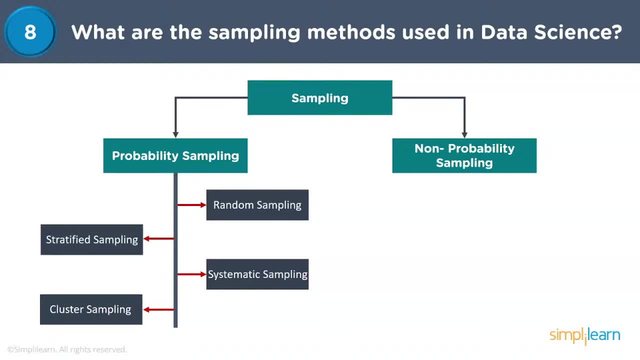 as random sampling. So in random sampling every individual is chosen entirely by chance and each member of the population has an equal chance of being selected. Then we have stratified sampling. So in stratified sampling, subsets of the population are created based on a common 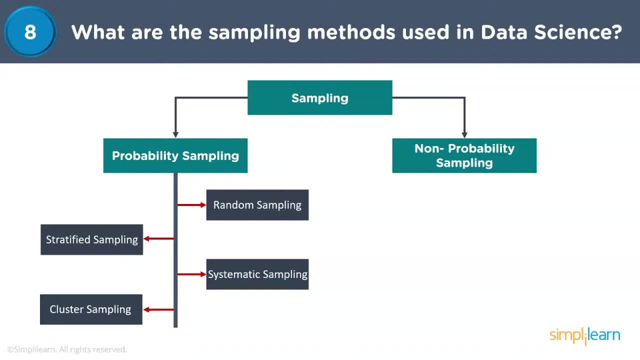 factor and samples are randomly collected from each other. Now talking about systematic sampling. So in systematic sampling, a sample is created by setting an interval at which to extract data from the larger population. An example could be selecting every fifth row in a spreadsheet of 100 items and creating a sample size of 20 rows for analysis And 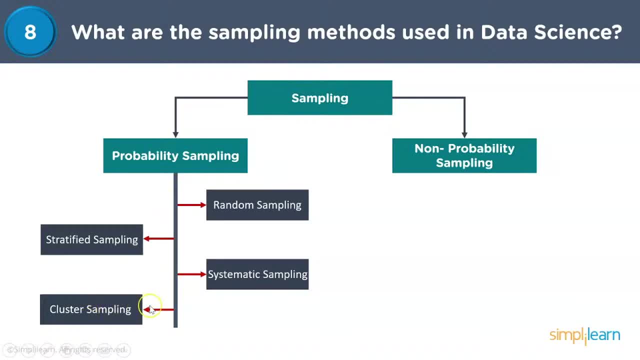 finally, under probability sampling we have cluster sampling. So in a cluster sampling subgroups of the population are used as the sampling unit rather than individuals. So the population is divided into clusters and a whole cluster is randomly selected to be included in the analysis. 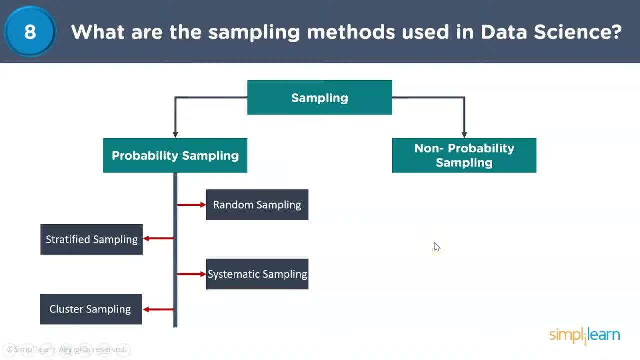 Now let's look at the sampling methods that are present under non-probability sampling. So first we have convenience sampling. So for convenience sampling, the samples are selected based on the availability. So this method is used when the availability of samples is rare and costly. So based on convenience, samples are selected. 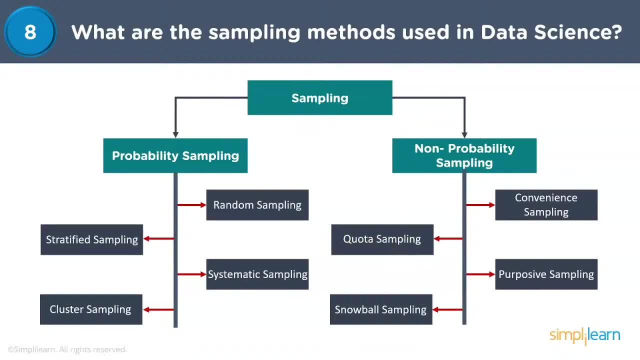 Second, we have quota sampling. So quota sampling depends on some pre-set standard. the proportion of samples in the sample should be the same as the population. Next we have purposive sampling. It is also known as judgmental sampling. You select members of sampling on the basis of the objective of the study. It is very useful when you want. 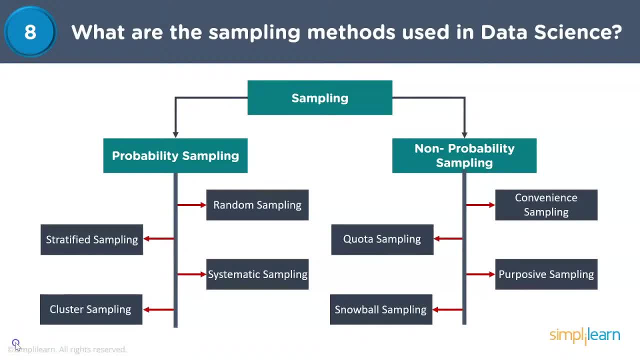 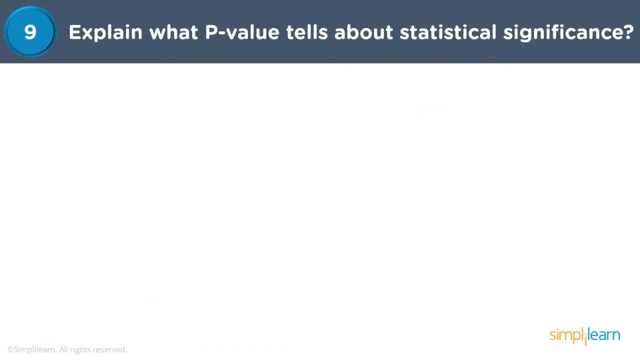 to reach a particular or targeted sample quickly. Finally, we have snowball sampling. So the snowball sampling technique is used in situations where the population is completely unknown and rare. Let's move on to the ninth question in our list. So explain what p-value tells about. 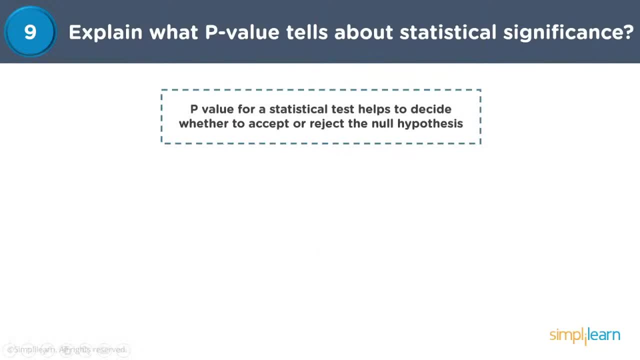 statistical significance. So p-value is a statistical test that is used in hypothesis testing. It helps you to decide whether to accept or reject the null hypothesis. The null hypothesis, represented as H0, is a commonly accepted fact. It is the opposite of alternative hypothesis. Researchers and 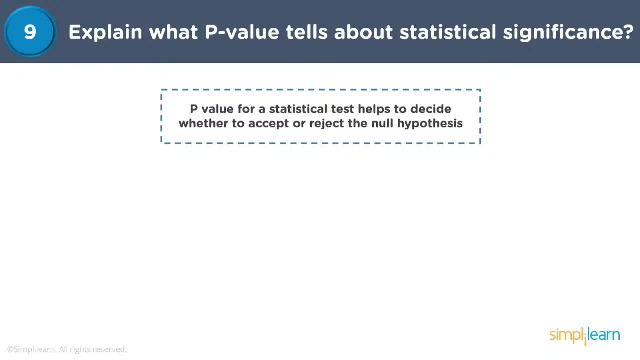 scientists work to reject or disapprove the null hypothesis. They come up with an alternative hypothesis that they think explains a phenomenon and they work to reject the null hypothesis. For example, null hypothesis or H0 could be the world is flat and an alternative hypothesis could be the world is round. 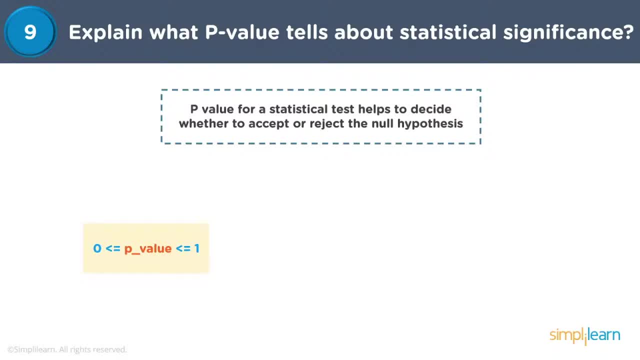 So the lower the p-value, the greater the statistical significance of the observed difference. Now, the p-value is just one piece of information you can use when deciding if your null hypothesis is true or not. The p-value, like the null hypothesis, is very important. You can decide. 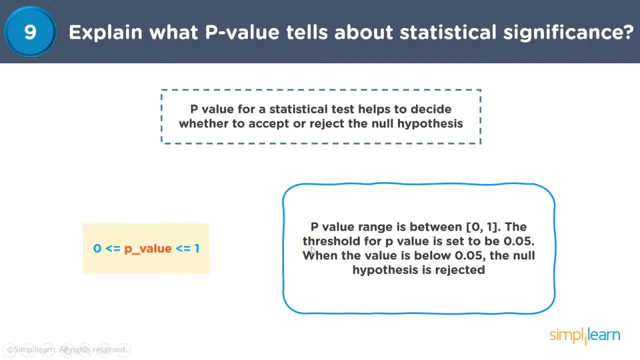 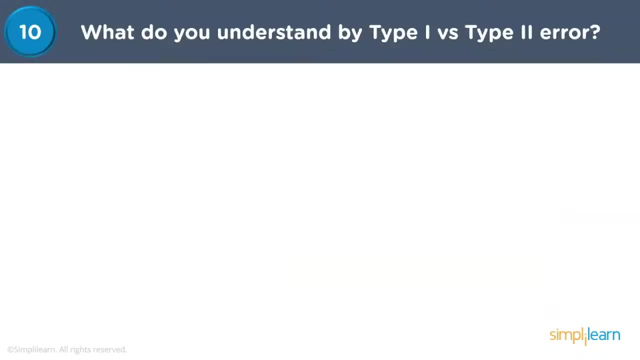 between 0 and 1. as you can see here, the threshold for P is set to 0.05. when the value is below 0.05, the null hypothesis is rejected. now coming to the final question in our list of mathematics interview questions for data science. so 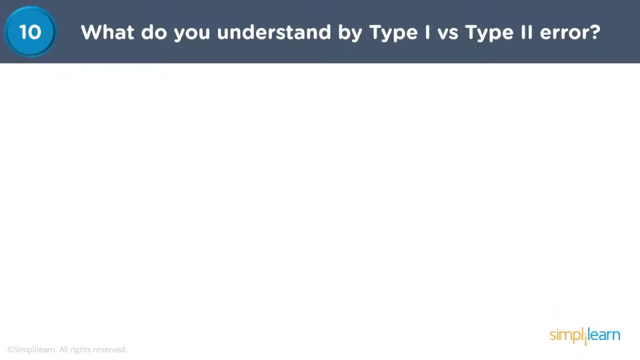 the question is: what do you understand by type 1 versus type 2 error? now, in statistical theory, the idistical error is an integral part of hypothesis testing. in statistical hypothesis testing, no test is ever 100% certain. that's because we rely on probabilities to experiment, even though hypothesis 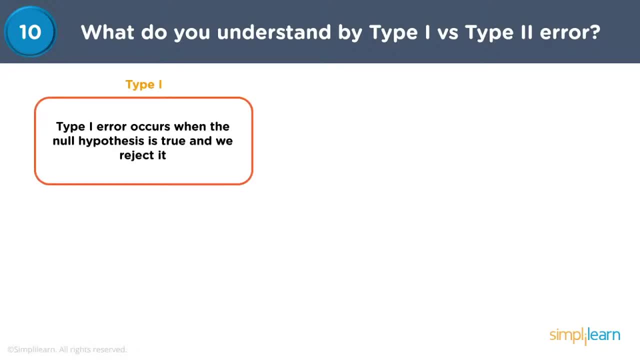 tests are meant to be reliable. there are two types. so type 1 error occurs when the null hypothesis is true and we reject it. it is also known as a false positive finding or conclusion. an example could be: an innocent person is convicted. and type 2 error occurs when the null hypothesis is false and 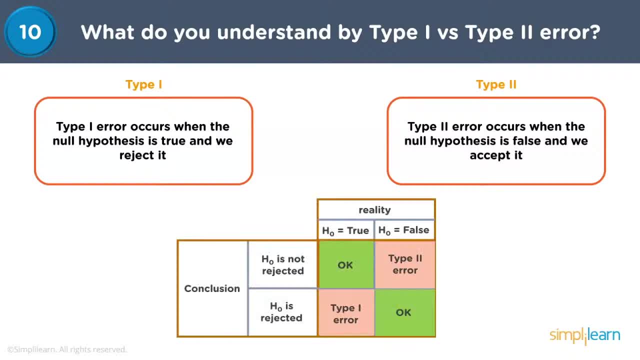 we accept it. it is also known as false, negative finding or conclusion. an example could be: a guilty person is not convicted. so here you can see, we have a reality where your null hypothesis is true and here we have the null hypothesis is false, and this is where the type 1 error lies. so this can also be.